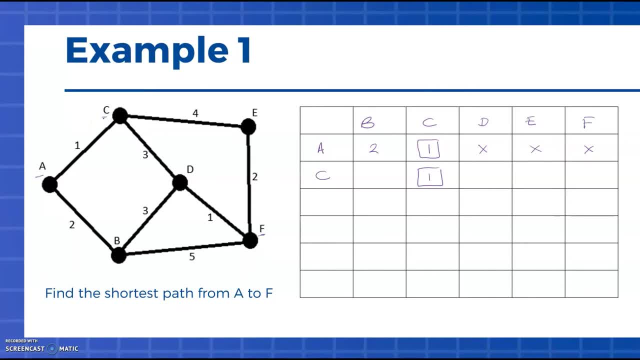 our starting point, if you like. so we have traveled from A to C and we're now seeing what's the next shortest connection. So at this point a couple of little admin things. I like to cross out or blackout the rest of that column for C. There's no need to keep revisiting it. 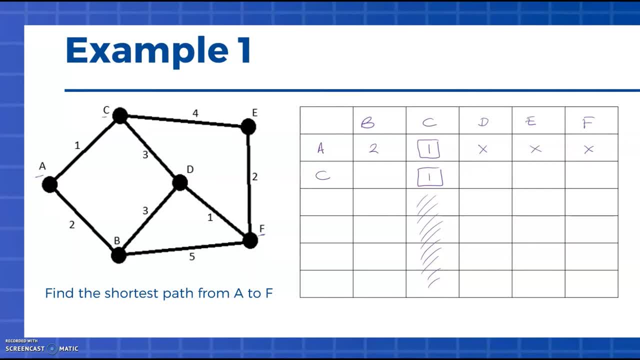 We've identified the shortest way to get there And so from now we're looking at C, So the pathway from C to B. there is no direct connection, so we take the pathway from directly above that. So we take that two and bring that down. We. 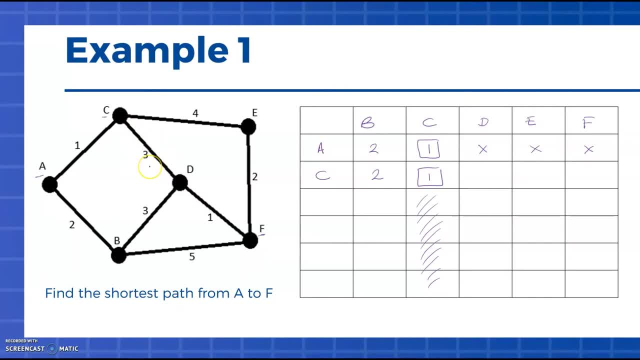 look from C to D. there is a pathway that is worth three, but we had to travel one already to get to from A to C, So we're actually looking at from A to C to D. in total that pathway was four, So we write down four as that distance. 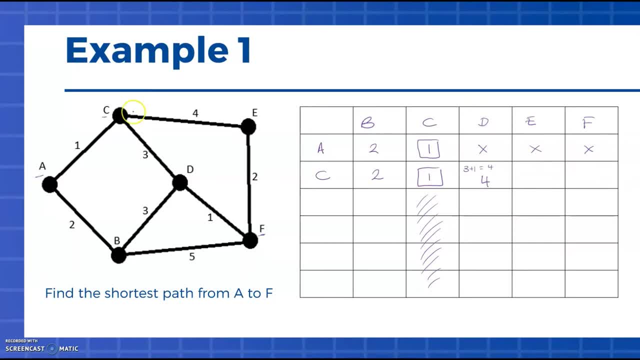 that journey, C to E, again C to E, there is a pathway of four, a direct connection, and we add the one from the box. So we add that value A through C to E gives us a pathway of five And F. there's no direct connection from C to F. So again we bring down what was. 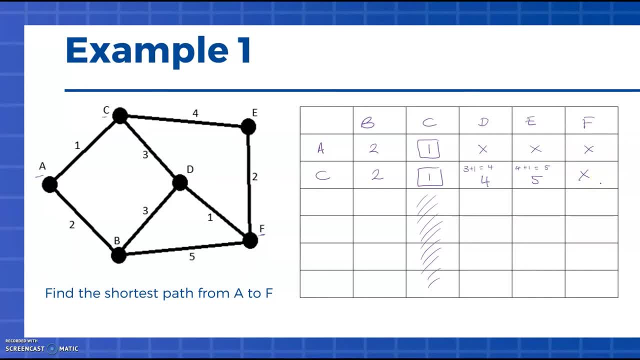 above. In this case that was a cross. there was no pathway yet, And so now we repeat, We look for the lowest value in that row, And so here that would be the two. We bring the two down, and we bring vertex B down as our next start point. I. 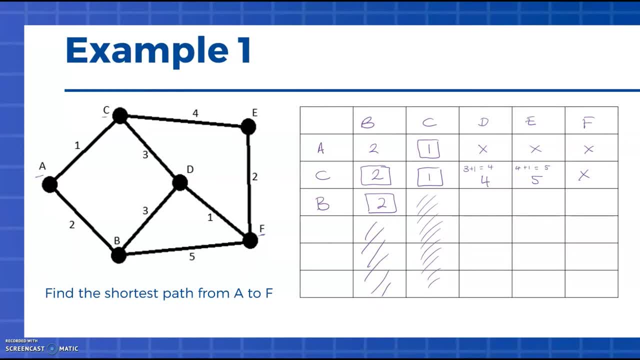 can get rid of that rest of that column B. So now from B we're looking at a pathway to D. There is a direct connection. That's three. We have already travelled two units to get to B, And so that gives us five as our pathway. This is where we have to stop and say: well, what was the? 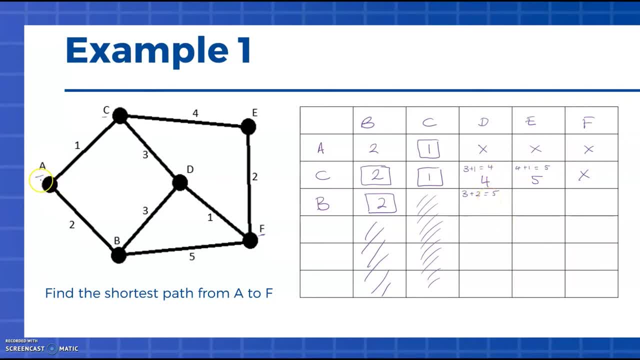 shortest way of us to get from vertex A to vertex D, And at the moment we're seeing here that the pathway through C is actually shorter than the pathway through B. So we look at these two values and we take the smallest of the two, So four becomes our value. we note down here. It's all about checking. 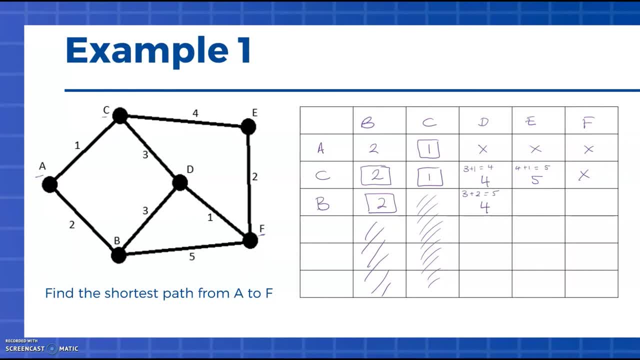 well, what was the smallest or the shortest way of getting to that point through the vertices that we've already covered? So we keep moving along. B to E: there is no direct connection, So we take the value from directly above, B to F. 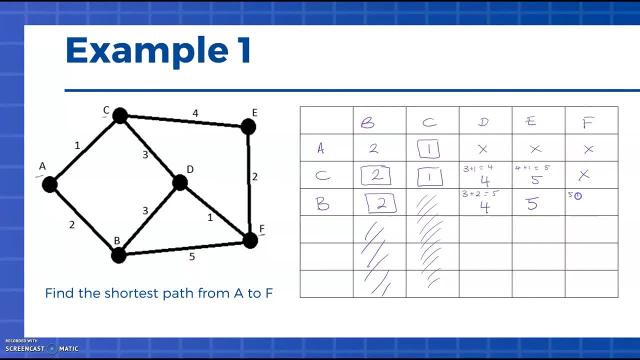 This time there is a direct connection Where, if say, as the numbers open for the final extension or five, we already travelled 2 to get there. So we're at 7 now, as we wrote, we right down 7. Again, now we stop, We look for the lowest value, which is the 4.. 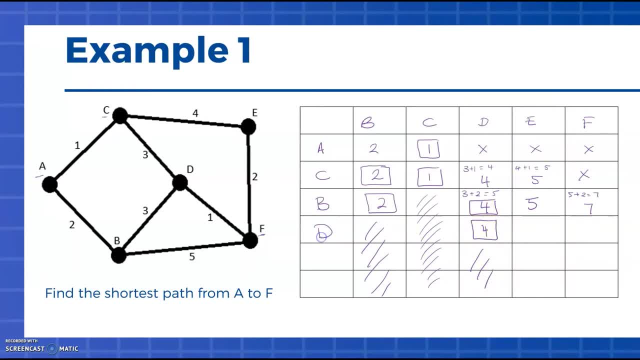 So we bring our 4 down, We bring vertex D across here, And so D is now our starting point. From D to E, no direct connection from above. d to f, we have a connection. that is one, and we already traveled four, so five again. we 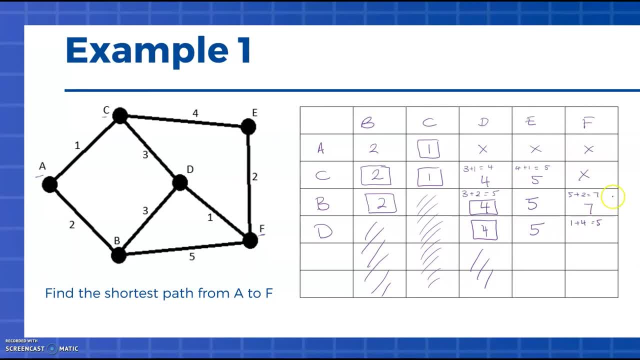 check and compare. five is smaller than our previous distance we had for f, so we write down five. now at this point, here i have two vertices giving me, or two pathways that are giving me the same distance. it doesn't matter which one i choose, i will eventually end up with the same answer. 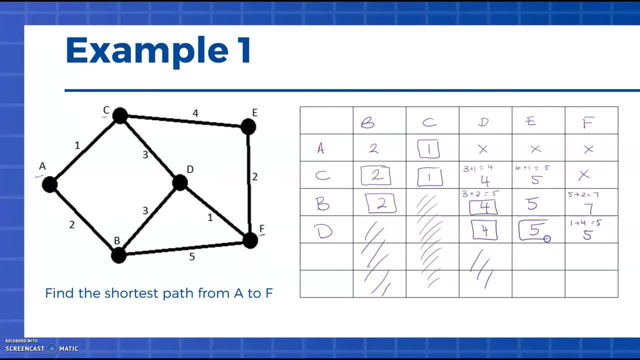 so choose whichever one you like. i'm going to go with e. so i bring down my boxed five, i bring e across as my starting point, and so from here i'm at vertex e. to get to vertex f, i've got a pathway of two. if i already traveled five, that would give me seven, but in this case 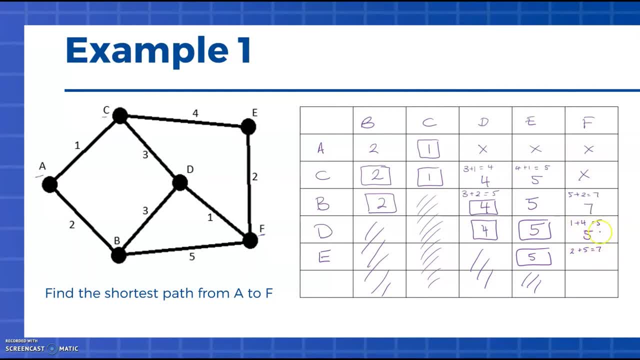 i've set up five and i've got a pathway of two, and i've got a pathway of two and i've got a. there is a shorter way of getting there, okay, and so five fired our vertex. D from above means that now I'm at my finish point, I am at F, and so at this point, 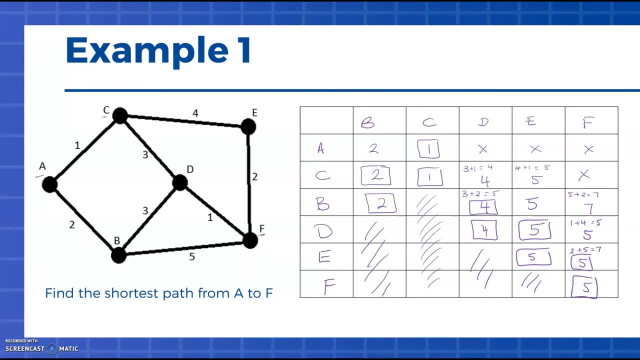 here. I've done all of the background work. now it's about, or how to identify what is the shortest path. and what other information does the table give me? okay, so the first thing that the table is giving me is the pathway there, so the distance or the weight of that pathway, and so if we look at this final value, 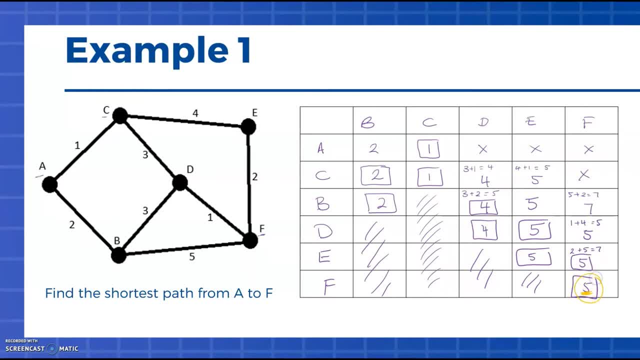 here this five. that is the weight of our shortest path. okay, so we know the weight of our shortest path is five. how we identify what the pathway is is by looking at our table. where is now backtracking, starting at the end? so I'm starting here in this column for vertex D, and then I'm going to go back to the 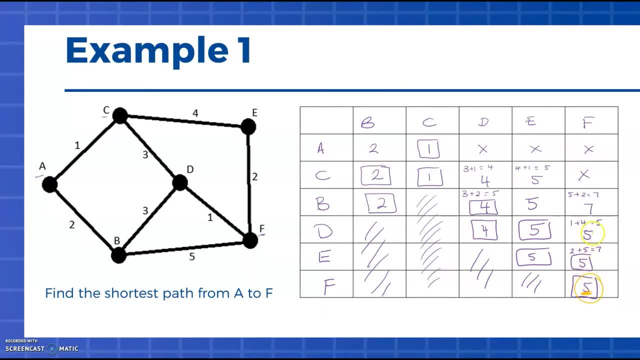 vertex F and you'll notice that some of the values are five and we reach a point where it then changes back to seven. so we're just going back as far as our last five and then we're going to look across to see what row, what vertex that came. 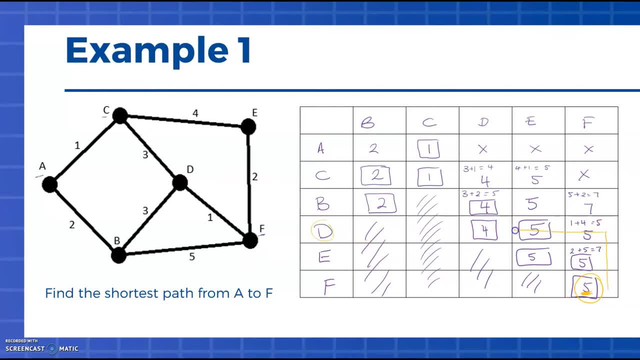 from. so it was vertex D, so I'm going to shift across to the column that lines up with D, and now I'm looking at the number four. so I'm going to keep going up until it's no longer a four in the bottom row, and then I'm going to go back to the 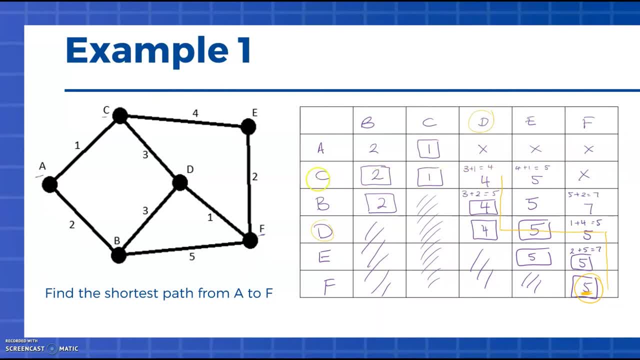 box. so this is the last four that lined up with vertex C. so again I look at where is column C, and now I'm working with the number one, and so again, I'm going to go up until there's no more ones, which gives me back to vertex A and 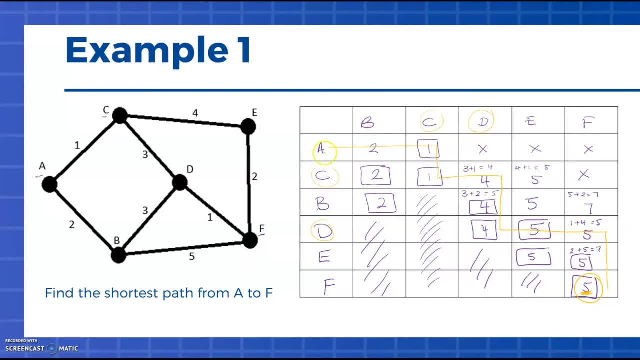 if I just look at the horizontal lines. okay, so A C, D, and then I'm going to go back to D and finally to F, A, C, D, F, and in my graph, A C, D, F. that is my shortest path and it adds up to five that I have in my final box. I should always check. 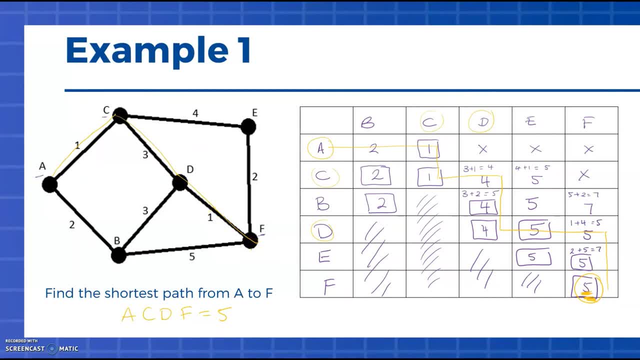 that on the graph and make sure it matches. but if you've done your algorithm correctly, you've done your calculations correctly in the table you will end up with a four in the bottom row and then I'm going to go back to the box. so this is the last four that lined up with your path and the weight matching. 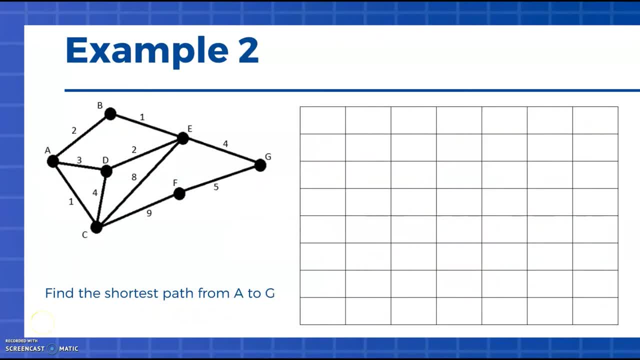 the shortest path in your graph. okay, so this time, next example, looking at the shortest path from A to G in this case. and so again, first steps. we always put our first vertex in that first or the second row, the top of the table there, and we write the rest of our vertices across the top of the columns. so it. 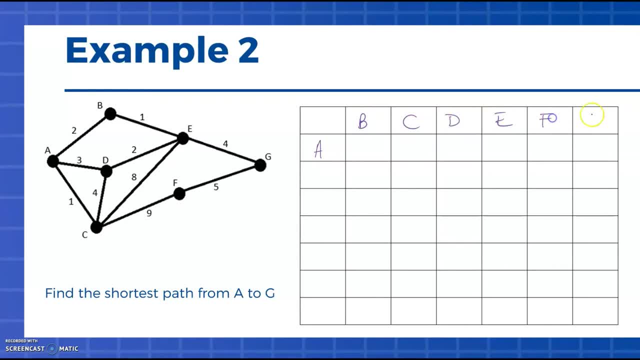 doesn't matter at the order, but we tend to do alphabetical order so that we can keep track, and now working our way through identifying each shortest pathway. so direct connections only. so, A to B, we have a pathway of two. A to C, we have a pathway of one. A to D: a pathway. 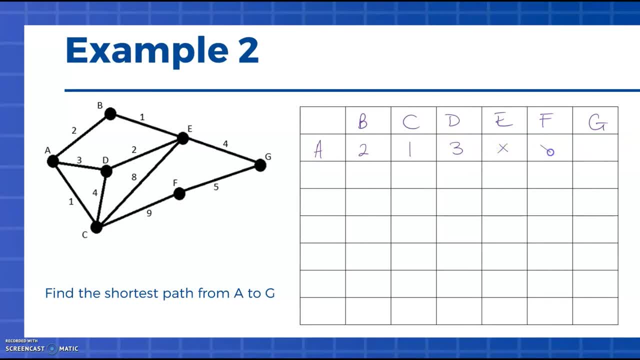 of three and no direct connection to E, F or G. so identify our smallest value, a shortest path, which was from C, the value of one, and then I'm going to go back to so we bring that one down and put c as our next starting point. so in our next row, 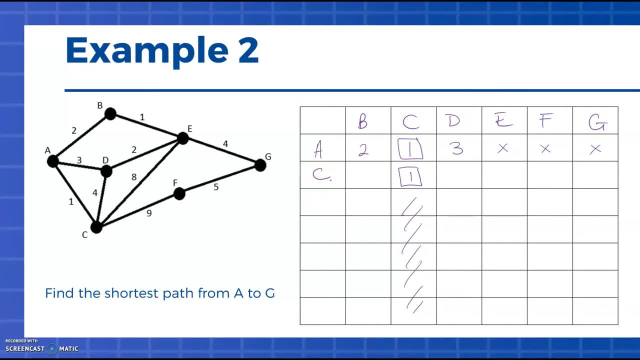 and so now, looking at c, c to a, we already know we had that pathway of one. c to b: there is no direct connection, so we bring the two down. c to d, we have a pathway of four. we already traveled one, so that gives us five. and here we stop and look and say: well, three. 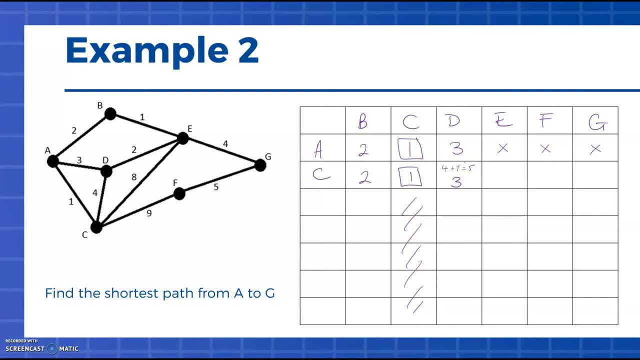 was smaller, so i'm actually going to bring that value down. c to e: there's a direct connection of eight plus the one we already traveled. so that means we're bringing nine as our value there. c to f: again we've got a value of nine direct plus the one we already traveled. 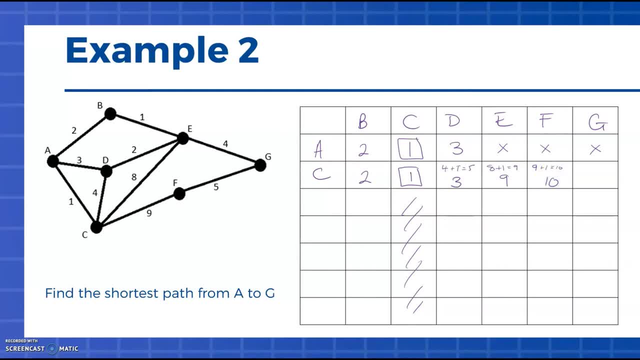 so 10 is our pathway and c to g there's no direct connection. okay, so b is our smallest number. so we bring vertex b down as our next starting point and bring our two down as our current pathway. so from b there's no direct connection to d, so we bring the smallest of the next value down. 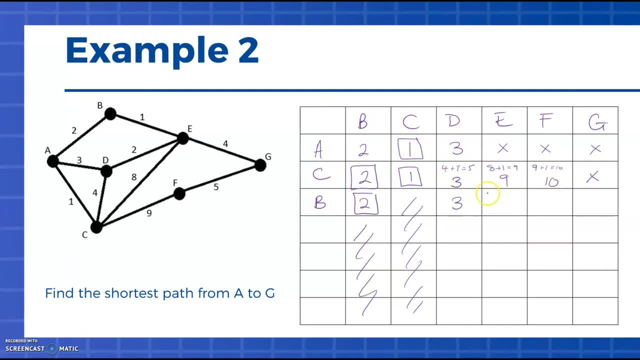 b to e. we have a pathway of four, so we bring that value down with our. doesn't matter exactly how long you immediately have it on the matrix. there's no direct connection. b to r, there's a somewhat odd value as a whole. so this is a volume ofteen, if we're looking at the third level. 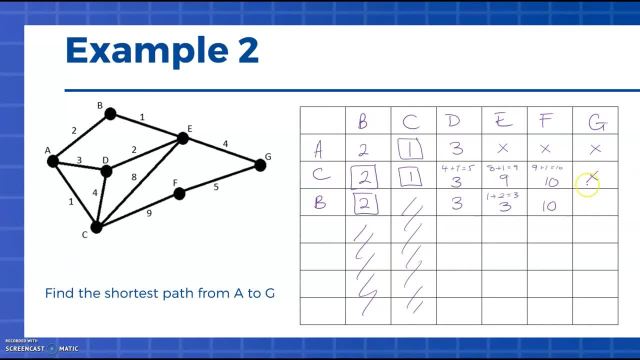 so it's a somewhat odd number and a somewhat odd number, so so we bring the. This time we're going to choose the one that's not directly immediately to the right of what we've already done. So I'm going to take E just to show you that it can work that way. 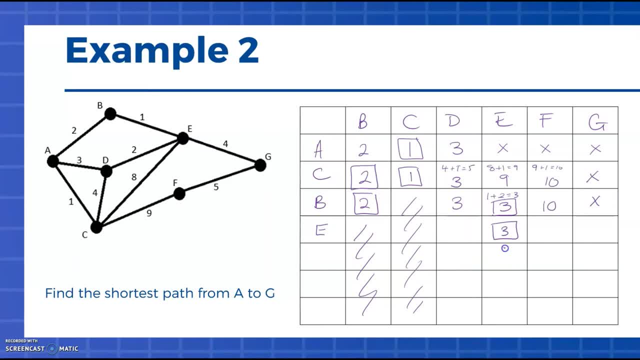 So we bring E across as our next vertex And we're looking at pathway from E to D. So E to D we have a pathway of two already travelled, three, which gives us a distance of five, But previously we've said three was smaller, was our shortest distance. 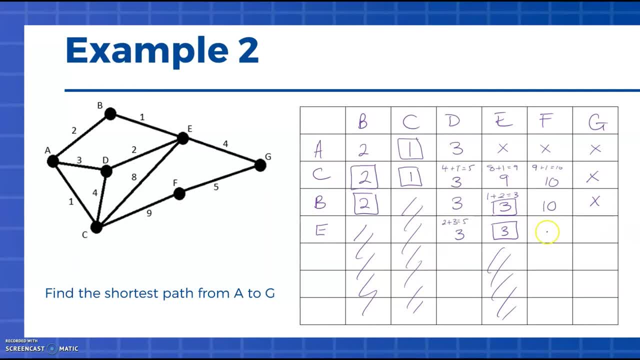 So we pop that down E through to F. there's no direct connection, So we keep the 10. E to G. this time now we have a connection, So that's a distance of four plus our box number that we've already travelled. 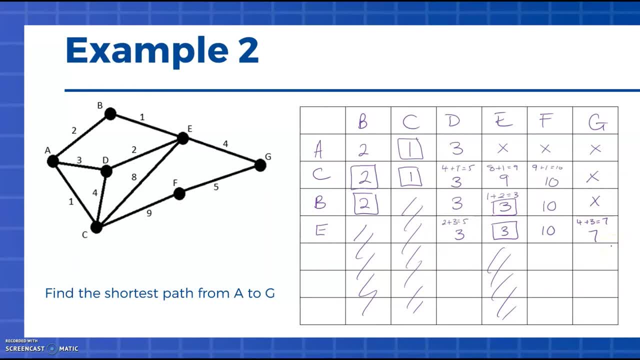 So that gives us a distance of seven, And so again our smallest number. we bring the three down, And D becomes our next starting point or focus point. Okay, so from vertex D there's no direct connection to F, So again 10 gets brought down. 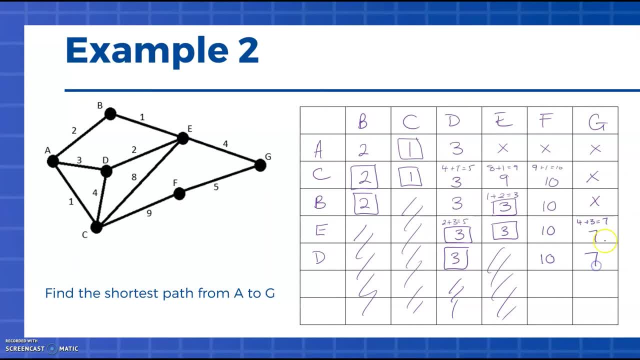 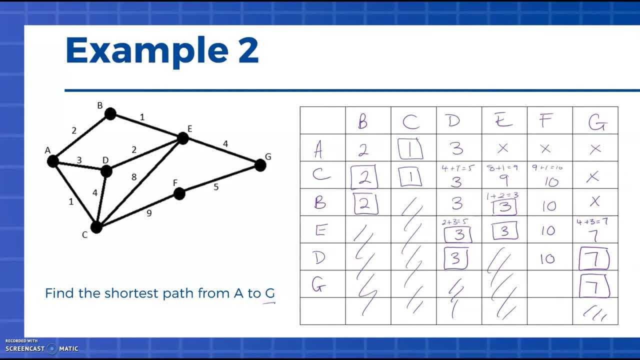 We've now hit our end point of G, So we can stop, And so this is where again, we would now look at our pathway. So, starting from our finished vertex of G, we start backtracking and go. well, if I'm working with seven, 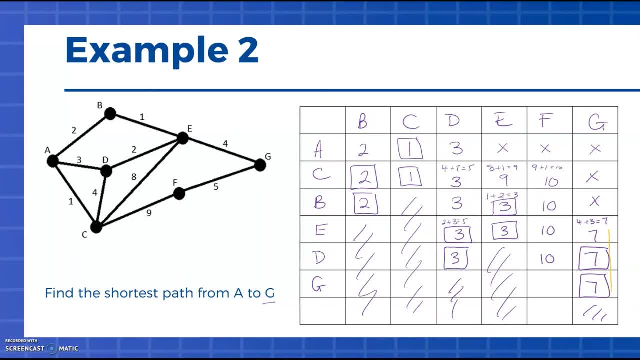 I will travel all the way up until I hit the last seven. When I look across, I'm at vertex E, So I'm going to go across to column E. Now I'm working with vertex E, number three. i go up until there's no more threes here. i'm at vertex b, so i'm going to come across. 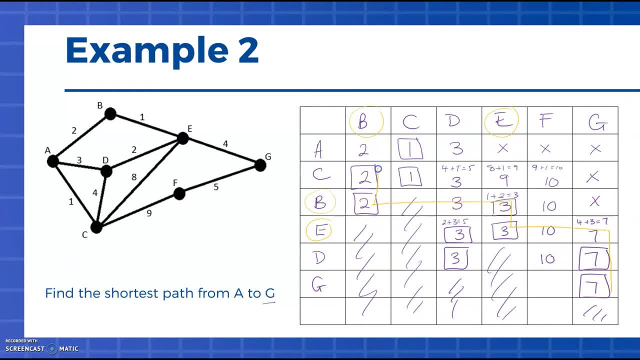 here and again. now i'm working with twos and i go until there's no more. twos means i end up back at my start point. so if i look at just my horizontal lines, i've gone from a, b, e to get me to g, so a. 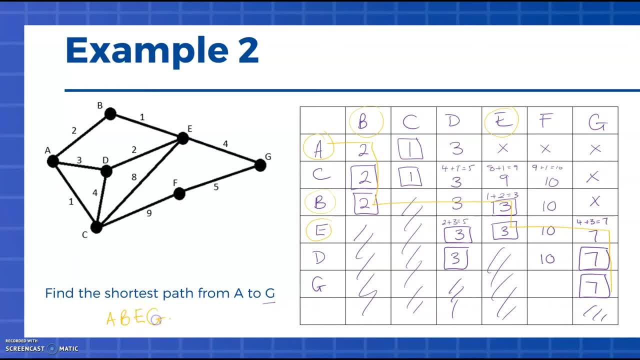 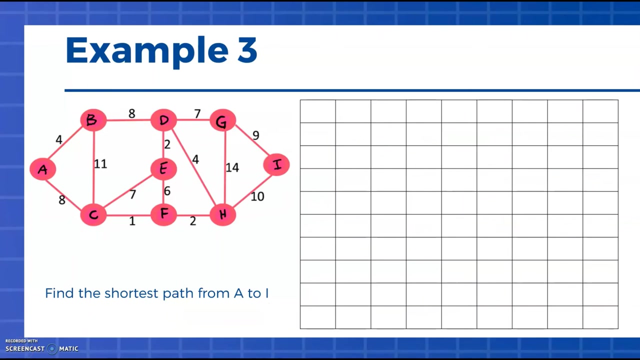 b, e to g and that pathway should equal seven in total. so let's check the graph: a, b, e, g, two plus one plus four is seven. so there's my shortest path and there's my weight of my shortest path. okay, one final example. so this is a bigger graph again, but the steps, even though there, 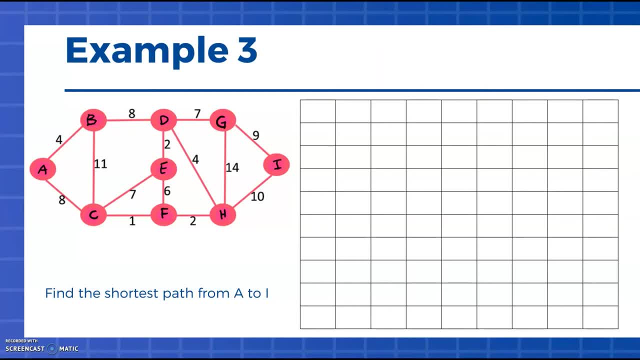 will be more steps required. they're no more complicated than what we have been doing, so it's just about repeating those steps constantly. so in this case i'm wanting to find a pathway from i through to- sorry, from a through to i. so if a is my starting point, i want to put that in that first row and let's just letter. 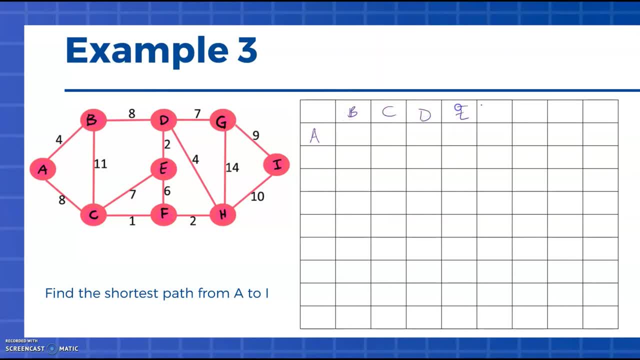 off the rest of the vertices. so you see d, e, g, h and i, and now again just working my way through. so from a to b, i have a pathway of four. from a to c, i have eight. there's no direct connection to d or e, f, g, h or i, so i only have two to start with. okay, so smallest number is four. 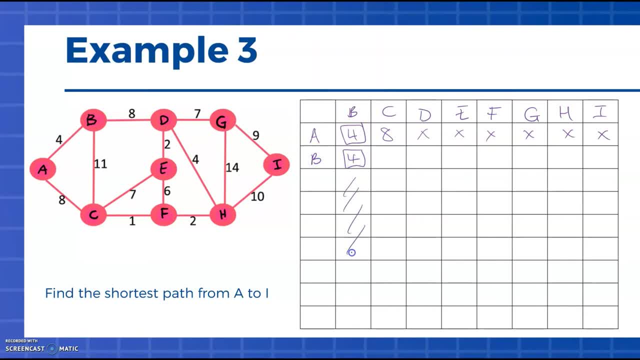 i bring down my four, and b is my next starting point, my next focus. okay, one final example looks a bit more complicated, but it's the same steps as what we've been doing previously. Okay, So this time we're finding the path from A to I. So remember, begin by putting your starting. 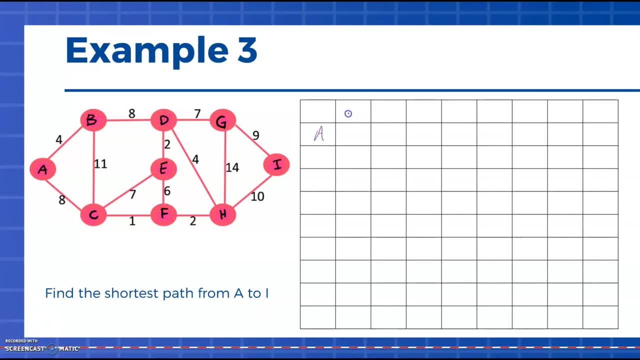 vertex. And it doesn't matter what order, but again, generally we just go alphabetical so we don't lose track. And now looking at each of our pathways, So A to B, we have a distance of four. A to C, we have eight. There's no direct connections for any of the other vertices from. 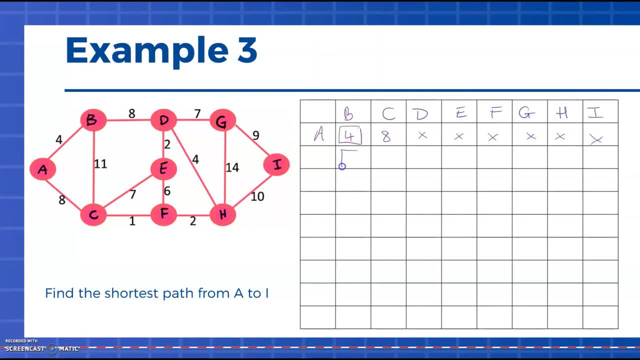 A, And so, looking here, our smallest value is four. So we bring down our boxed number, B becomes our next start point And we can disregard the rest of that row column. sorry, Okay, So from B, B to C has a connection of 11. And four would give us. 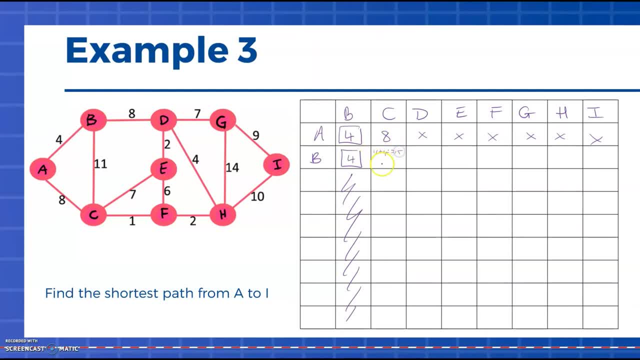 15.. But our previous pathway was eight, which is lower B to D. we do have a direct connection of eight plus our already travelled four, So which means we have a pathway of 12.. There's no direct connection to E, F, G, H or I again, And so now looking, eight is our smallest number, So we bring 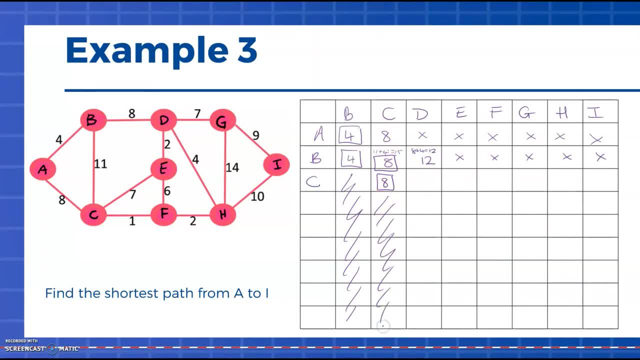 down our boxed C and we disregard the rest of that column. So we're now at C, C, no direct connection to D, So we bring down the previous volume of 12.. There is a connection C to E of seven plus the 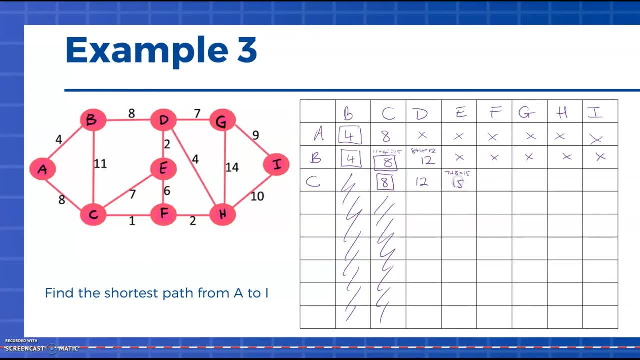 eight already travelled, So we have a pathway of 15.. From C to F there's a connection of one plus the eight travelled, So we have a pathway of nine. There no direct connection to G, H or I, And so now nine is our shortest pathway. So we bring down 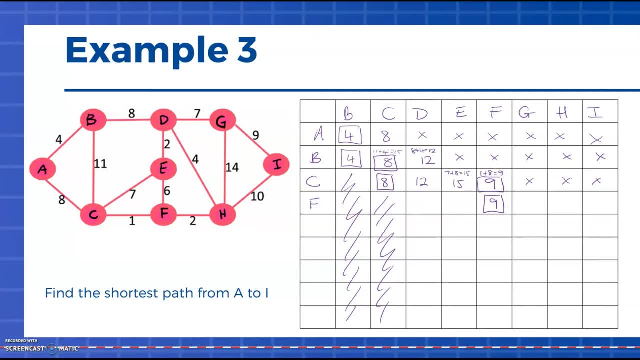 the nine, F becomes our next start point or focus point, And now we can go from there. So from F to D there's no direct connection. So again we bring down the 12. from above F to E, there's a. 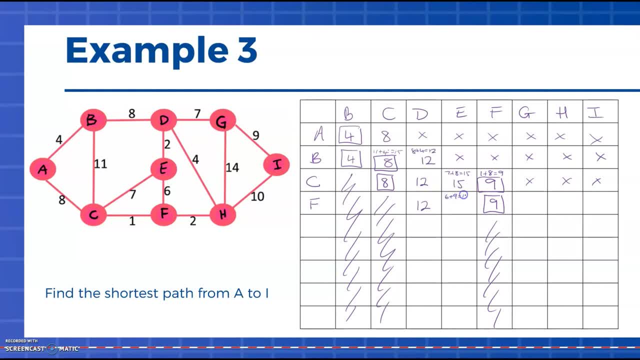 connection of six plus the nine already travelled, which gives us 15.. Same value as above. So we write 15 in the box. F through to G. no direct connection F to H. we have a pathway of two plus the nine. 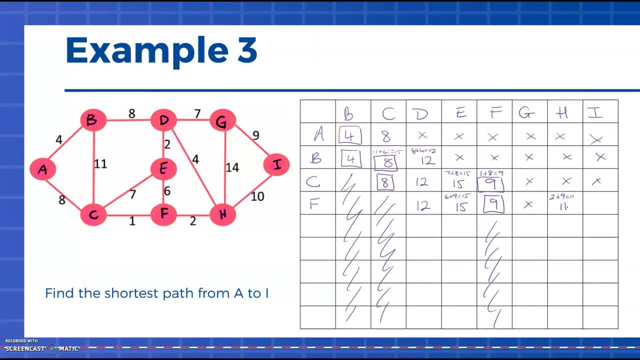 already travelled. So that gives us 11 there And no connection to I, And so now H becomes our smallest value. So we pick the 11 and H, the 11 in the box. H is my next row, my next vertex to focus on And work. 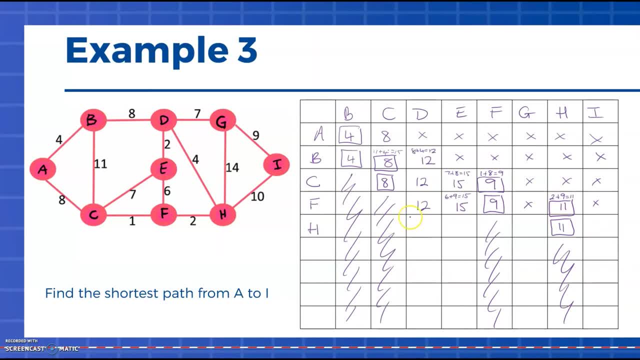 through what's left. So H to D, I have a pathway of four plus the 11 already travelled 15.. But I check above and 12 is smaller. So 12 is the value I'll bring down. H through to E: There is no. 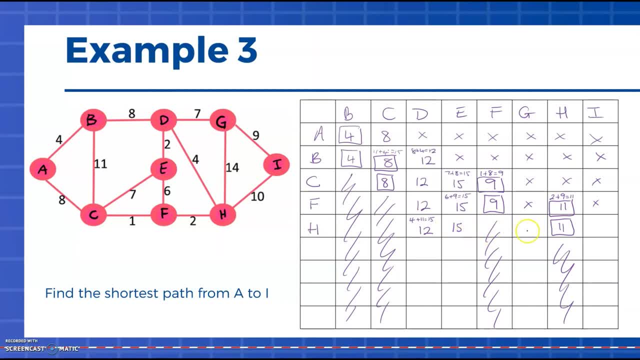 direct connection. So we bring the 15 from above. H to G. we have a pathway of 14 plus the 11 already traveled- okay, so 25. and h to i. i have a value of 10 and the 11 already traveled, so 21, okay. so again looking for the smallest value, which is 12. 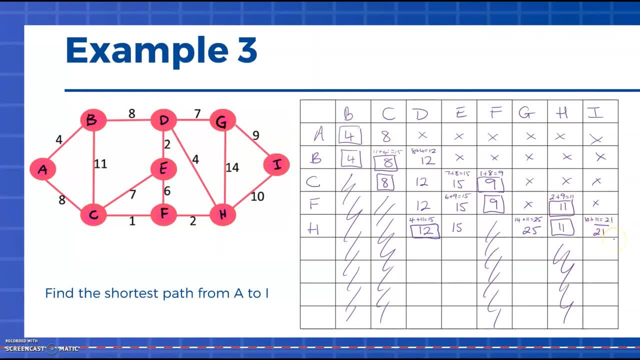 so even though i've finally got a connection to i, it's not my smallest value, so i need to keep working my way through this process. so now 12, which means i bring d down as my next focus and go back and look at d. so d has a direct connection of 2 to e and the 12 already. 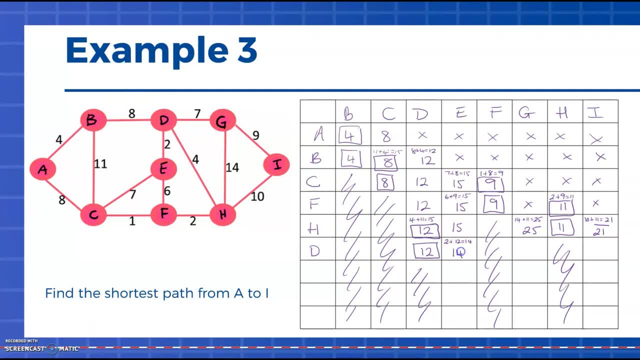 traveled 14, which is slightly less. so i bring 14 down as my next value. d to g: we have a connection of 7 plus the 12 already traveled, so 19, and again that's smaller than what's above. so 19, that's brought down here and d to i: no direct. 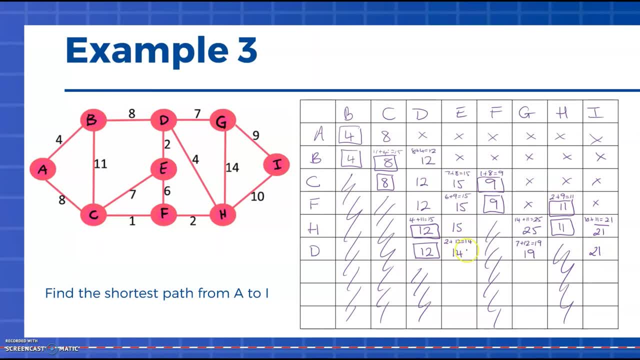 connection. so 21 comes down from above and 14 is the smallest value in this row. so again, bring my 14 down. i bring e across as my focus and you can see by crossing each of the columns out each time that it allows you to see. well, i only really have to check. 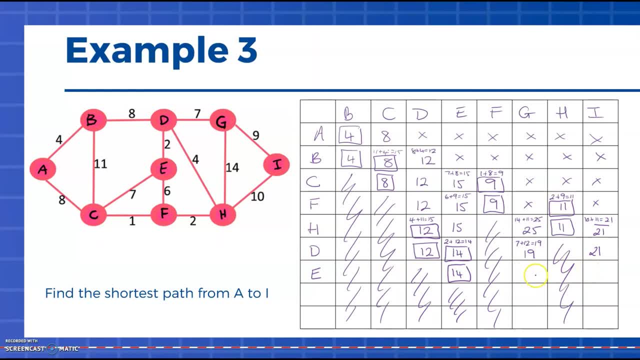 two pathways here, two vertices connections here, rather than checking them all again and sort of getting lost in what i'm doing. so from e no direct connection to g, so the 19 from above gets brought down. and again no direct connection from e to i, so 21, 19 is the smallest of those. 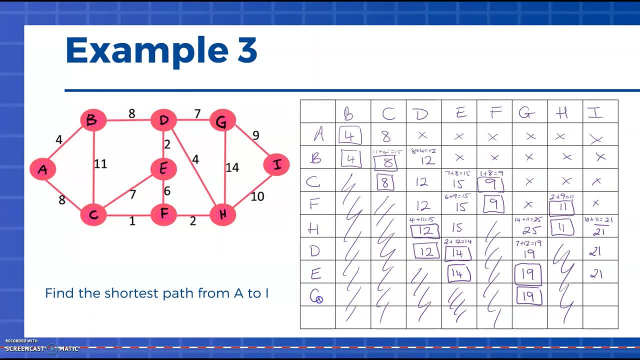 values. so i bring 19- g becomes my focus point, and i can get rid of that one- um g- to i. i have a pathway of 9 plus the existing 19, which would give me 28, but 21 is the smaller of those values, it's the only one left, and so that brings me to i, which is my finish point, that i 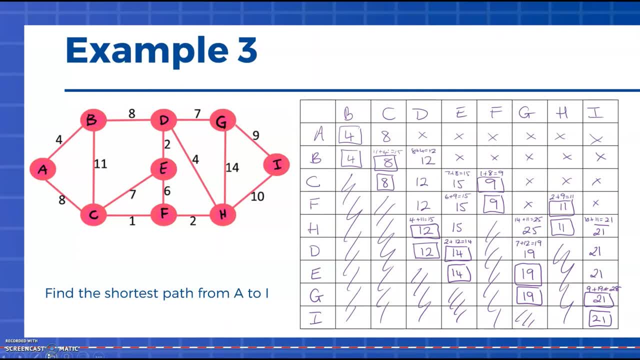 want to be at, and so almost there i've. now should have a pathway where the shortest path is 21. i can now identify from the table what is that pathway, and so let's just check that. and so remember backtracking. we start at the end, and so from this 21 i keep traveling up until the last 21. that is in line with vertex h. 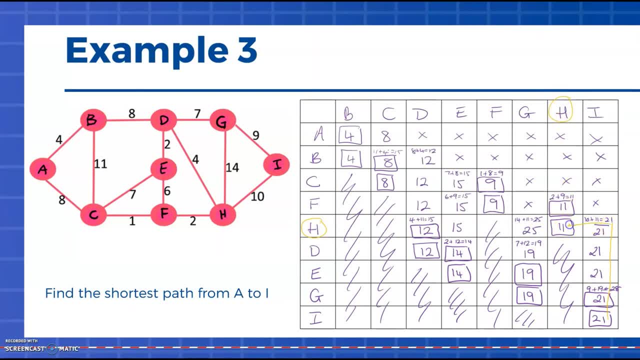 so i come across to h's column. now i'm looking at 11s, so i travel up until the last 11. that comes from f. i come across to column f. now i'm looking at nine. again, that comes from c. so i'm going to go across to column c looking at the number eight. i travel up until there's no. 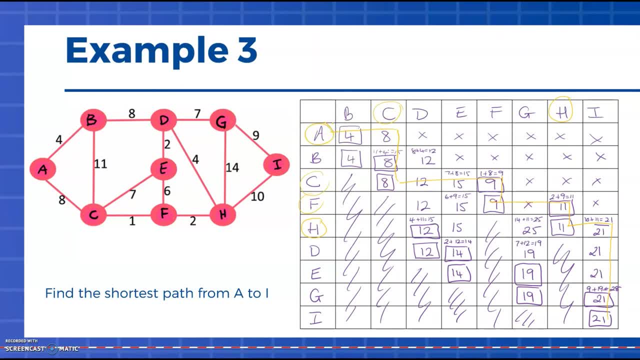 more eights. and here i am back at my start, point a. so looking across at the horizontal lines, i'm going from a to c, f, h, i. so a, c, f, h i. it should give me a path of 21 and we want to check that out. 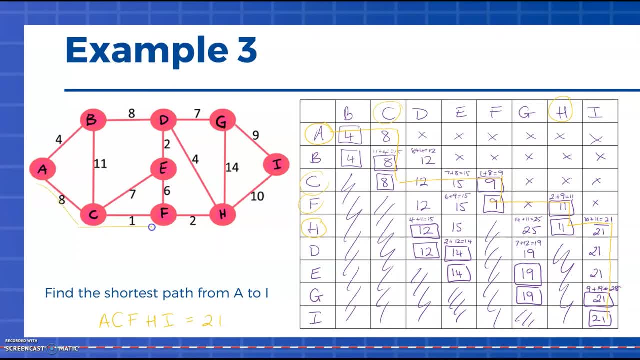 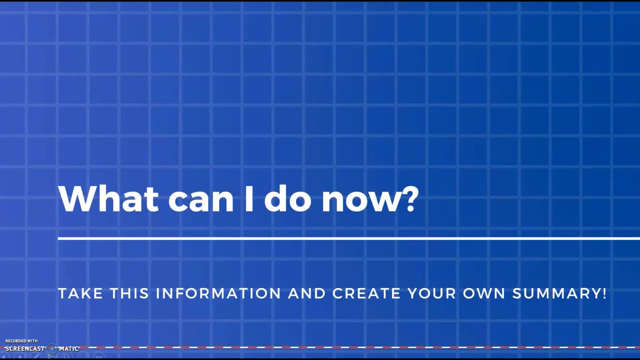 now on our graph. so a, c, f, h, i and eight plus one plus two plus ten is twenty one. so there's my shortest path. okay, so that's it for the examples. i suggest you work your way through a couple more examples. get some notes down that will.